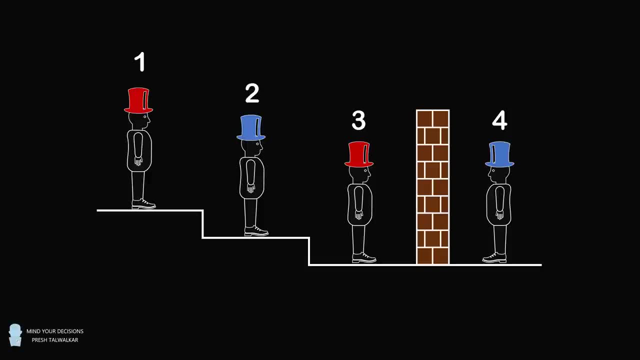 prove it. So he lines up the four logicians as follows: We have one, two, three all facing forward, then a brick wall and then on the other side of the brick wall is logician four. The warden says I'm going to place two blue hats and two red hats on the four of you. They all know. 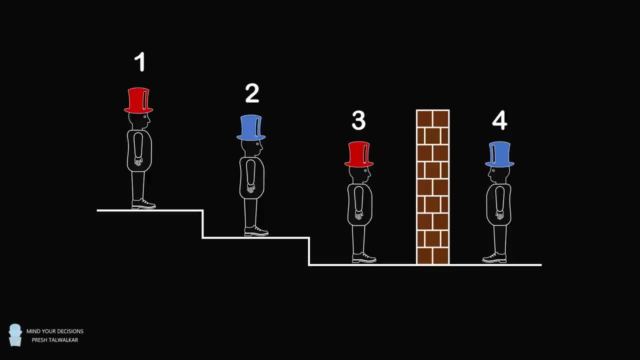 these rules. They're only allowed to look in front of them. There's no cheating. They're not allowed to take their hats off, They're not allowed to talk to each other and they're not allowed to do anything else. They have to figure out the answer using pure logical reasoning. 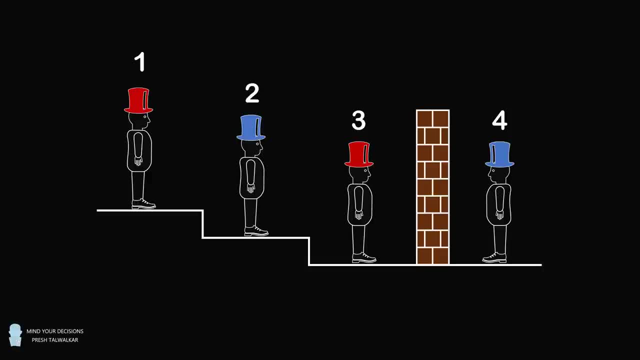 The warden says: I'm going to give you some time. If any one of you can state the color of your hat with certainty, I will let you all out for free, Being perfect logicians. none of them will speak out of turn and just guess. They will only speak if they know the answer for sure. So the question: 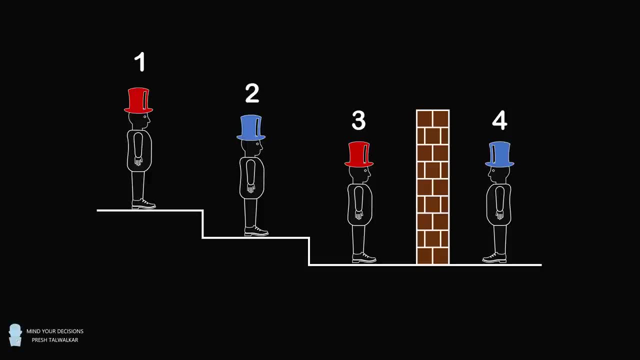 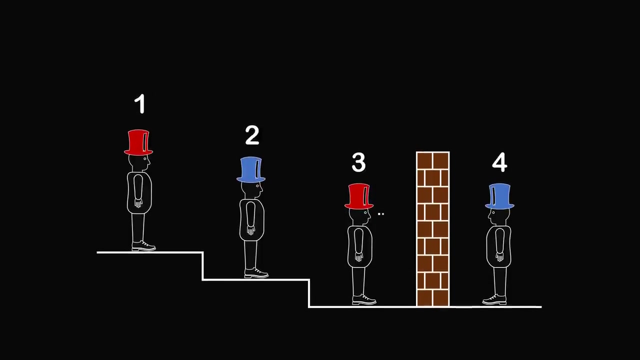 is: can the four logicians be freed and how would they do it? Pause the video if you'd like to give this problem a try and, when you're ready, keep going. Keep watching to learn how to solve this problem. So how can we work it out? First, logician three only looks at a brick wall, So there's no information. 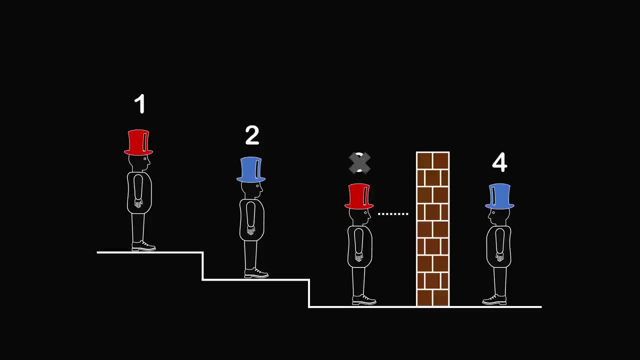 that the third person could have. There's no way this person could shout out with certainty. The same thing is true for logician four. The logician only sees a brick wall and doesn't have answers. so four is not going to shout out any answers. 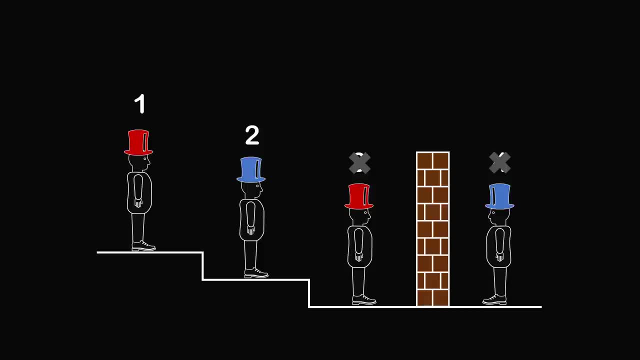 Now each of them is thinking there are two blue hats and two red hats. So there are, of course, four. choose two, which is 4! over 2!2! equals six different ways for the warden to arrange: two blue hats and two red hats on the four of them. 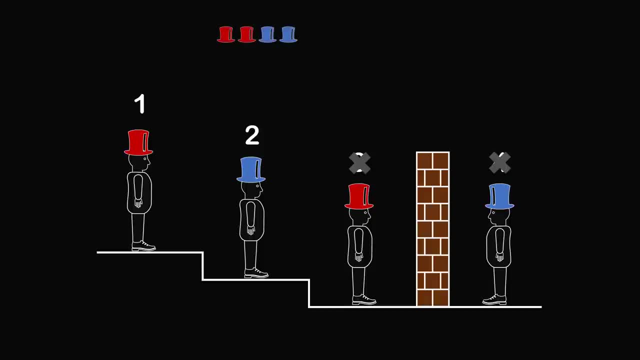 So they start thinking: what are the possibilities? It could be red, red, blue, blue, red, blue, red, blue, red, blue, blue, red, blue, blue, red, red, blue, red, blue, red or blue, red, red blue. 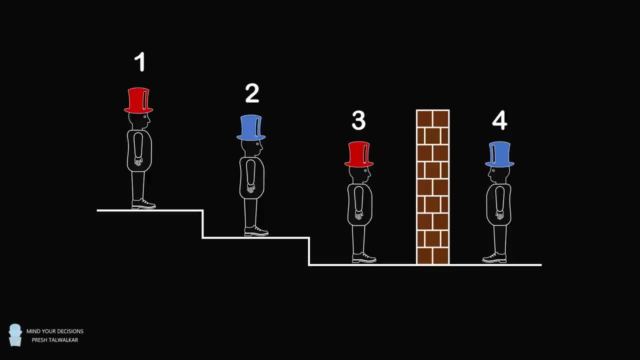 these rules. They're only allowed to look in front of them. There's no cheating. They're not allowed to take their hats off, They're not allowed to talk to each other and they're not allowed to do anything else. They have to figure out the answer using pure logical reasoning. 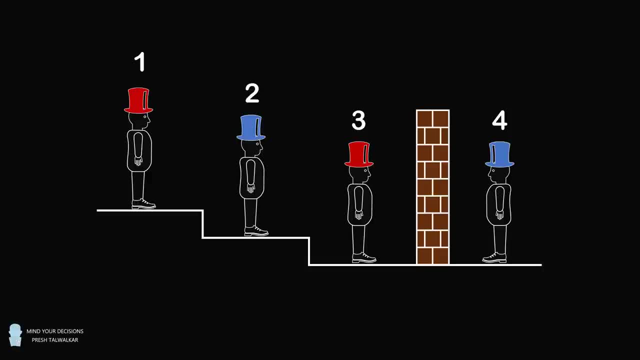 The warden says: I'm going to give you some time. If any one of you can state the color of your hat with certainty, I will let you all out for free, Being perfect logicians. none of them will speak out of turn and just guess. They will only speak if they know the answer for sure. So the question: 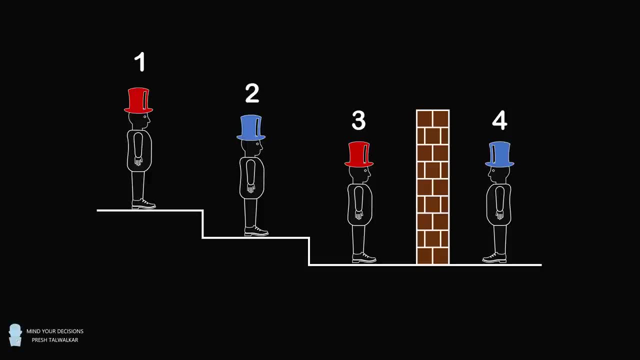 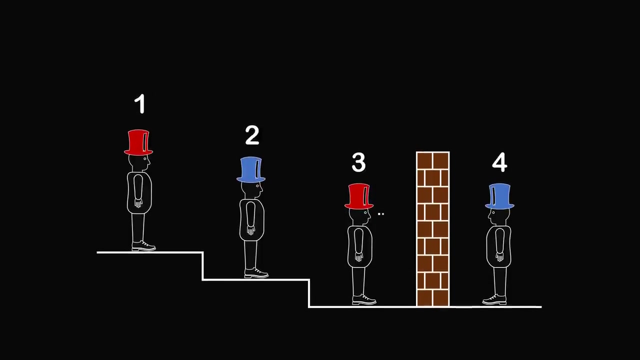 is: can the four logicians be freed and how would they do it? Pause the video if you'd like to give this problem a try and, when you're ready, keep going. Keep watching to learn how to solve this problem. So how can we work it out? First, logician three only looks at a brick wall, So there's no information. 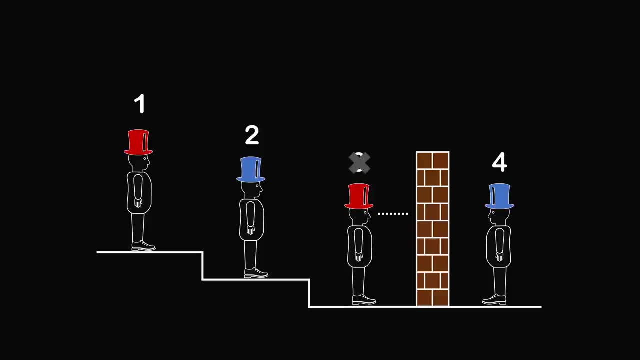 that the third person could have. There's no way this person could shout out with certainty. The same thing is true for logician four. The logician only sees a brick wall and doesn't have any answers. So four is not going to shout out any answers. Now, each of them is thinking. 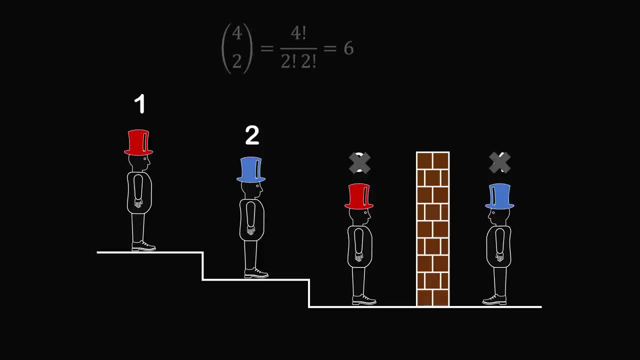 There are two blue hats and two red hats. So there are of course four. choose two, which is four factorial, over two factorial. two factorial equals six different ways for the warden to arrange two blue hats and two red hats on the four of them. So they start thinking: what are the possibilities? It could be red, red, blue, blue, red, blue, red blue. 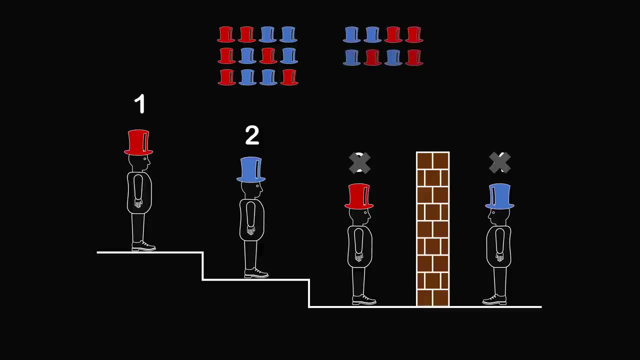 red, blue, blue, red, blue, blue, red, red, blue, red, blue, red or blue, red, red, blue. Now logician two sees a red hat on the third person. So logician two looks at which possibilities have: a blue hat on the third option. 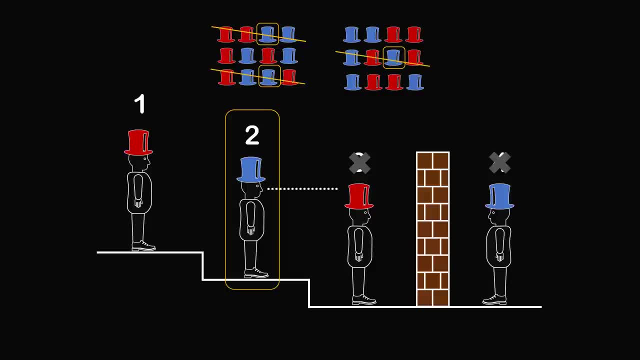 and says: these cannot be the possible arrangements. So we are down to three possibilities. Now logician one is also thinking the same thing, because logician one can see the hats on logicians two and three. So logician one not only knows they're down to these three possibilities.